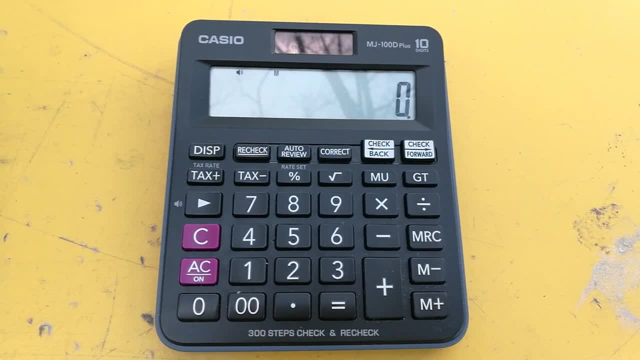 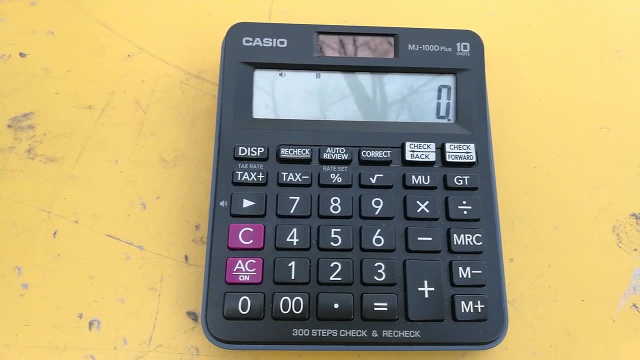 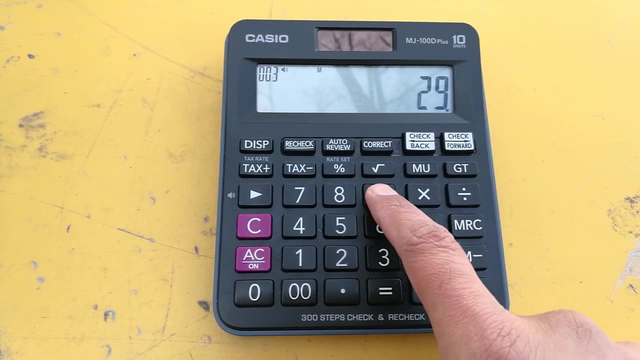 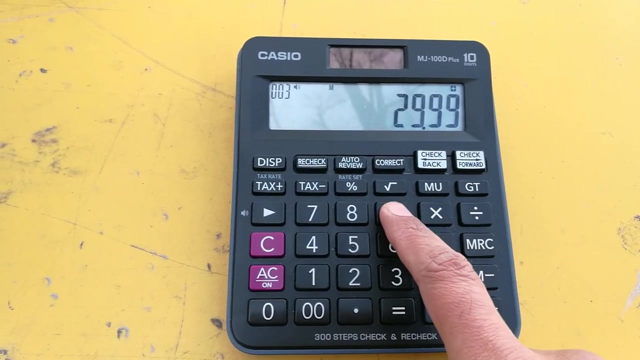 Hello guys, I hope you are doing really, really well. Today. I'm going to tell you how you guys can calculate the sales tax, guys. So first of all, for example, you have any product and the price of the product is, let's say, $29.99. plus you buy one more product, any product, and the price is $9.99.. So $29.99 plus $9.99, total will be $39.99.. 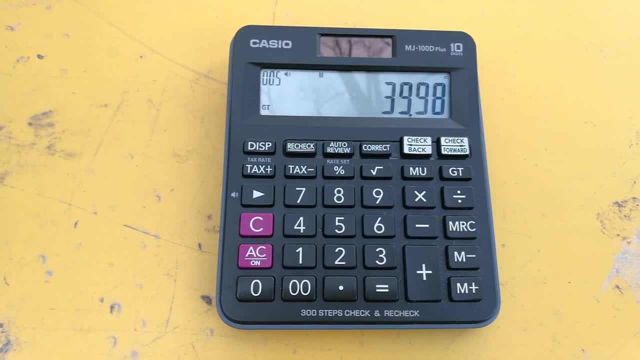 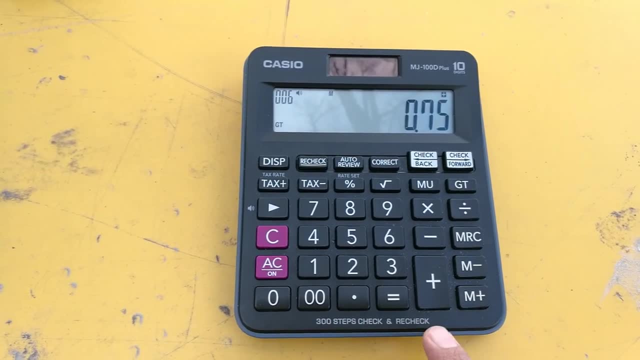 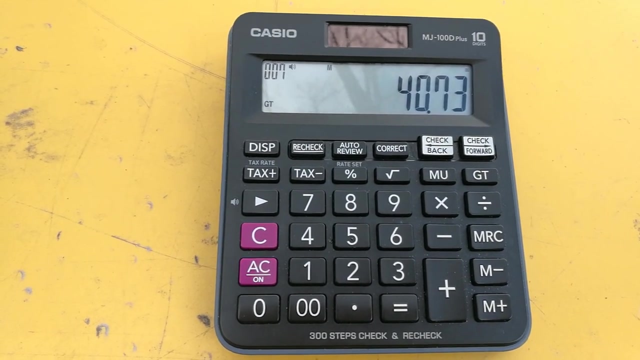 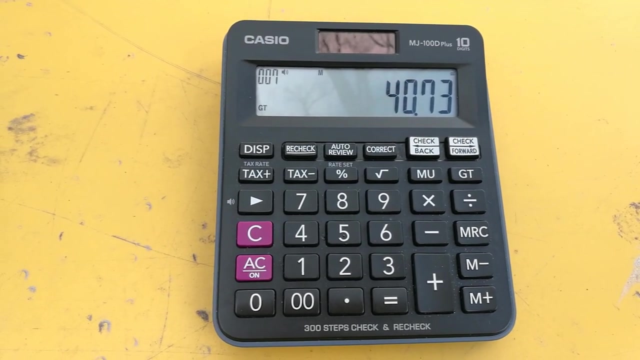 Guys, so $39.98.. Okay, and then you have a service charge, let's say 0.75 cents. Okay, guys. so the total altogether will be $40.73, or whatever the currency you have. guys. So now you want to calculate the sales tax. in different areas there are different sales tax percentage. So let's say we have a sales tax percentage let's say, which is very common, is 8.875%. 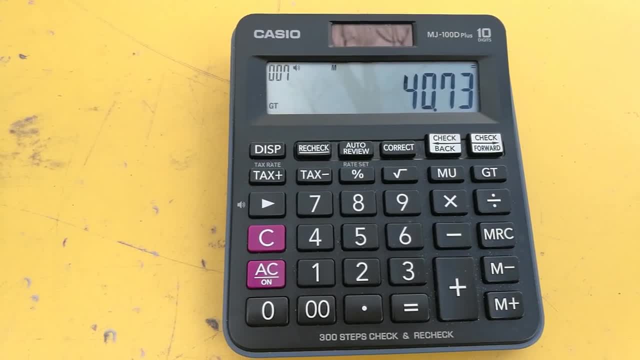 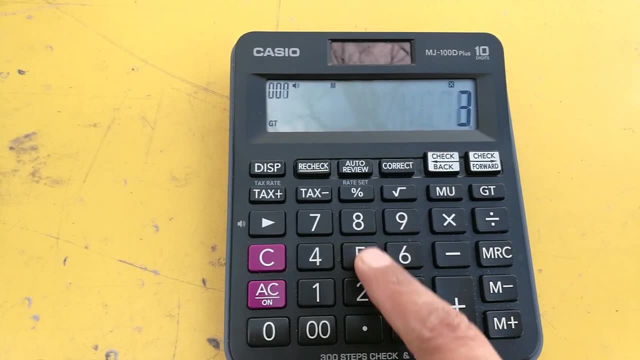 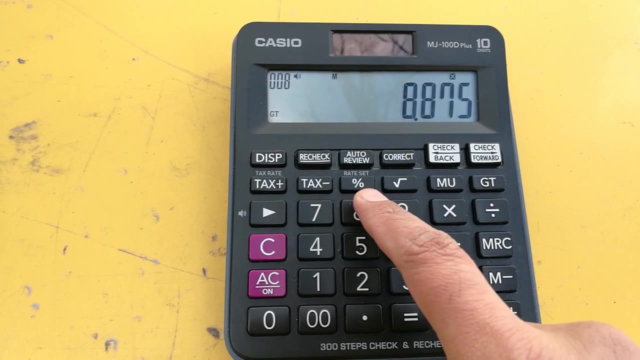 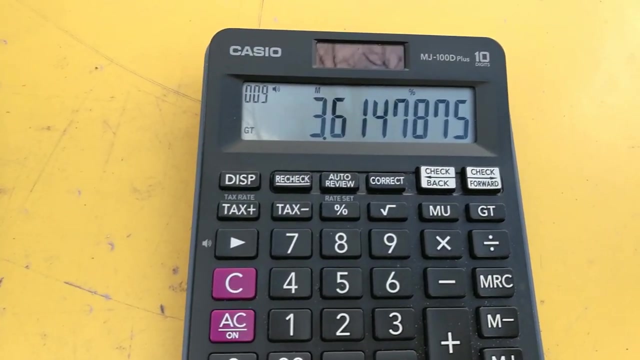 So what we will do now we have the total in front of us. we will multiply this, this amount. we will multiply it with 8.875.. Okay, guys, So when we multiply it and then we press the percentage button, this is the percentage button. guys. So when we multiply it and then percentage button, it come to us 3.61.. So $3.61 cents, guys. 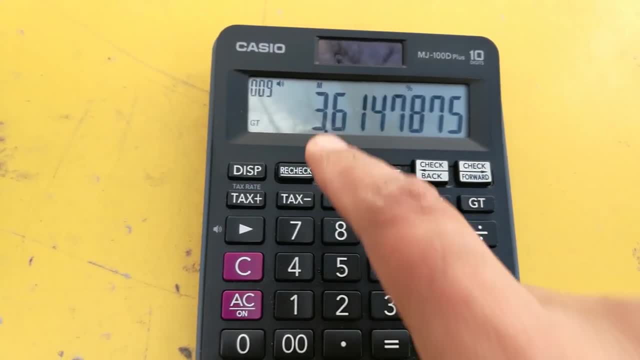 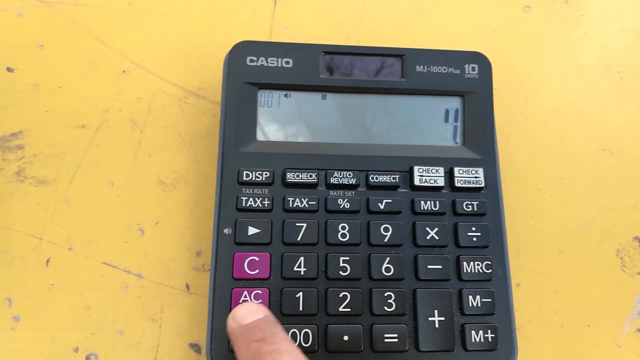 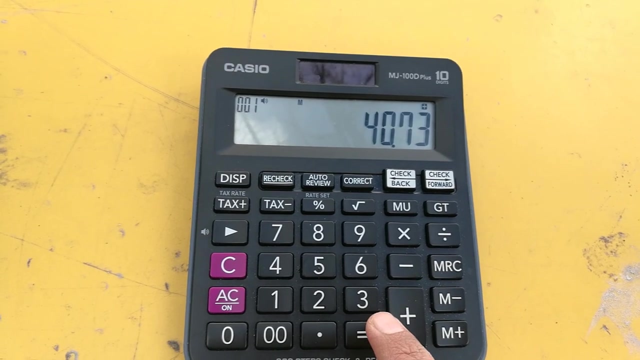 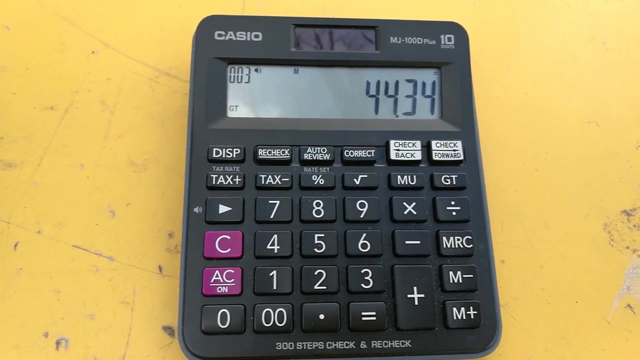 Okay, so this is the percent. Okay, now what we will do is we will add this one 40 point. sorry, 40.73 was our total and we want to calculate the sales tax. So we will add that answer: 3.61, $3.61 cents with $40.73 cents, So the answer is $44.34 cents including the sales tax, guys.